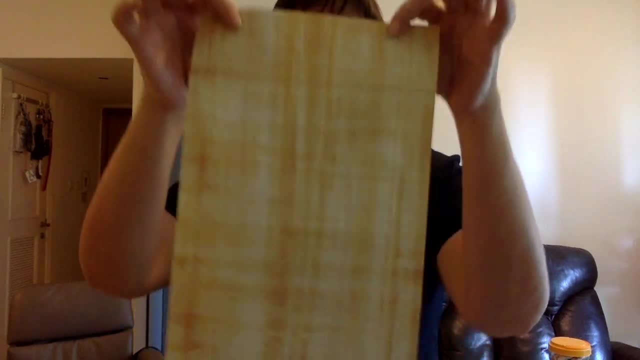 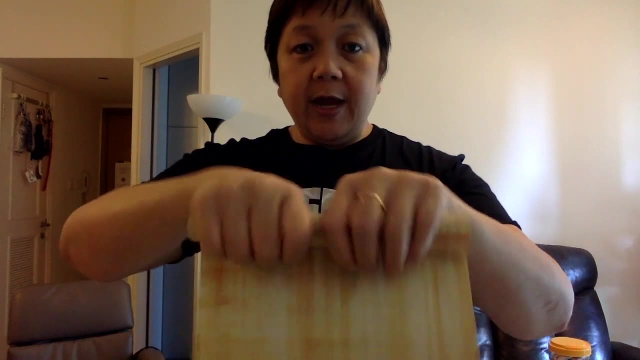 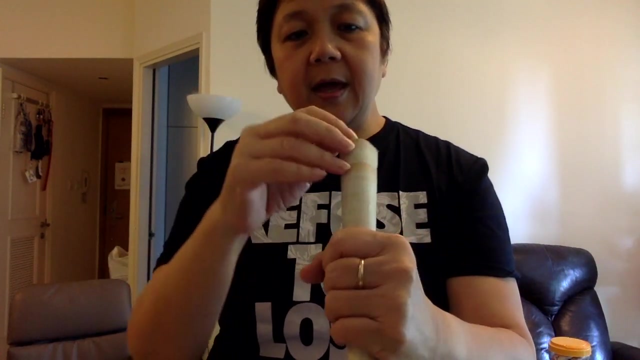 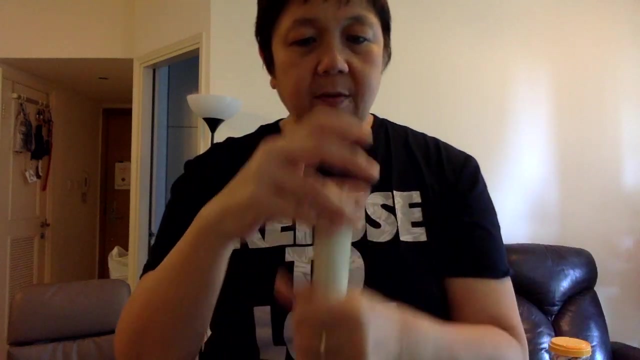 flute, you can roll it this way, but I can get more rolls if I roll it this way. okay, so I am just rolling. so just roll it, roll it, roll it and, okay, try to tighten it a little bit. okay, there you go, okay, okay. so before I did, 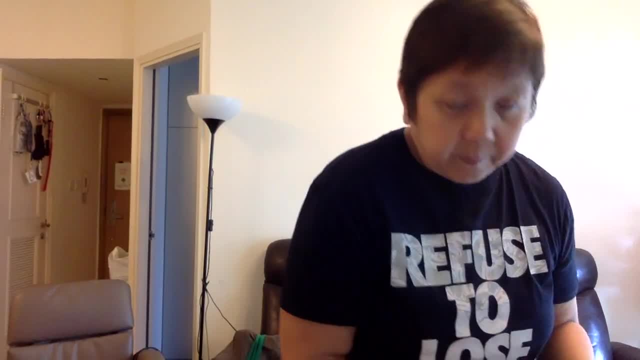 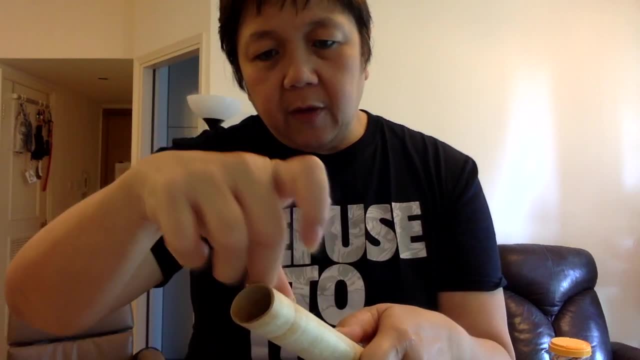 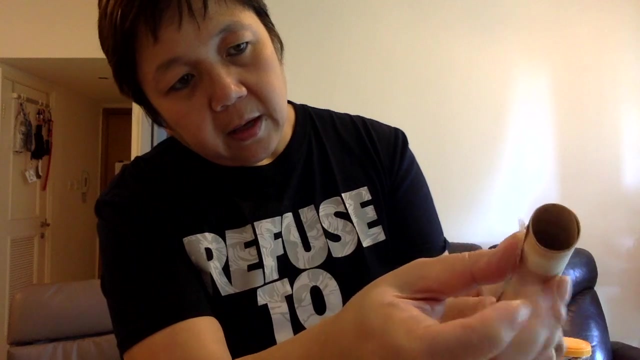 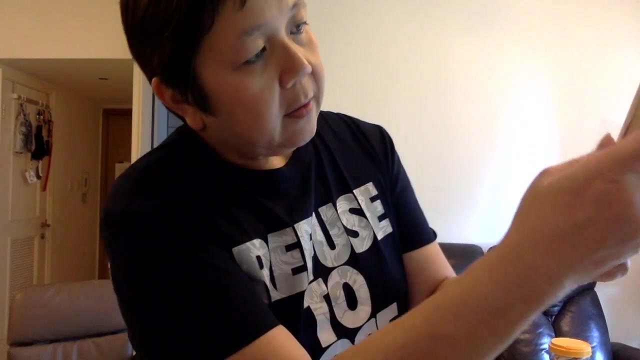 this: before I rolled it, I already cut some pieces of tape, okay, so that I can easily tape it together. okay, there you go. I'm just trying to put it at the very edge, okay, and there you have it. okay, so we have one down. okay, try to do the others. 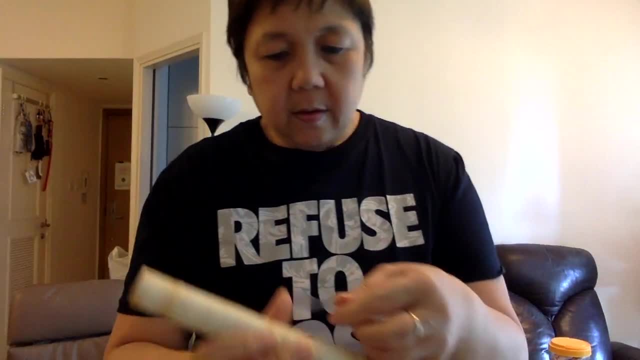 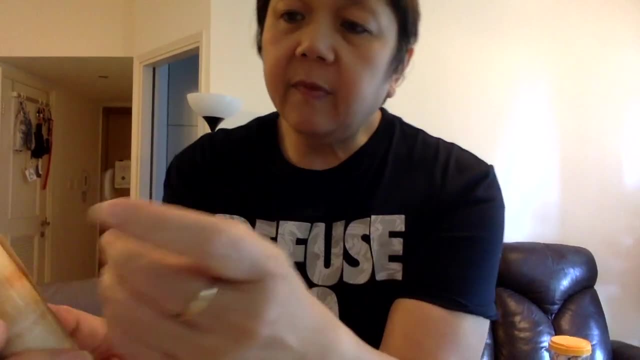 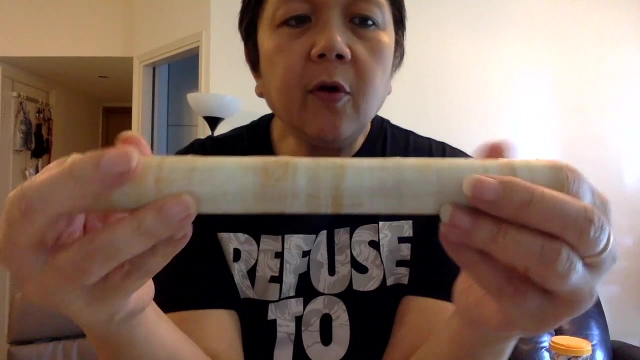 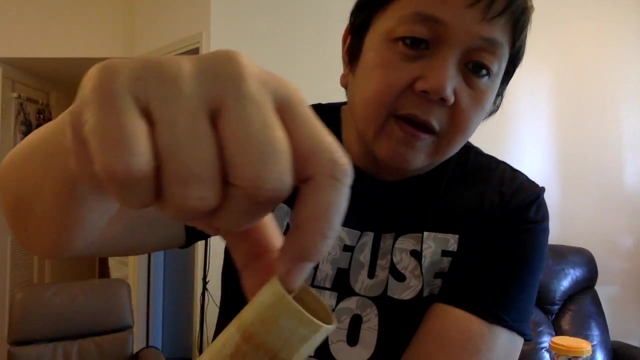 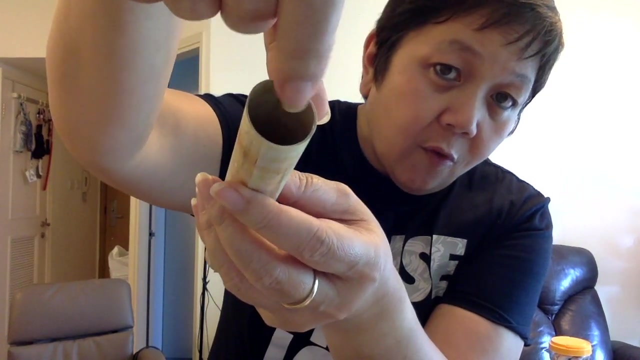 okay, and do the same so that you can secure the whole um seam. okay, there you go. I secured the whole seam with tape, okay, so the next thing you do is, if you look at the inside, you will see that there is this edge, unsecured edge. okay, you do not want to cut the hole over here, so you want to. 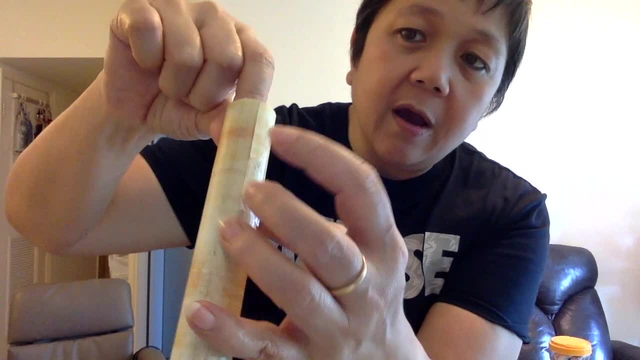 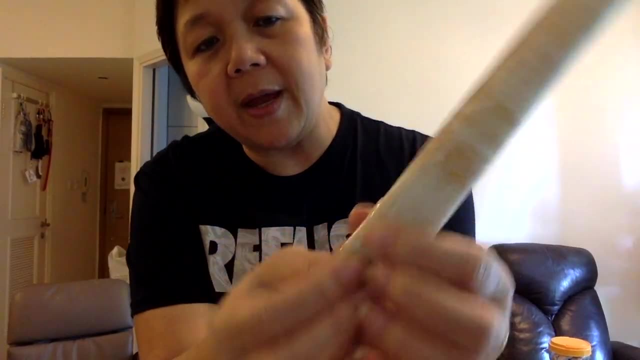 cut opposite it. so if this is the unsecured edge over here, I'm going to cut a hole on this side. okay, there you go. okay, there you go. okay if you did that side, okay. so what I need to do is I just need to bend it a little bit, okay, maybe. 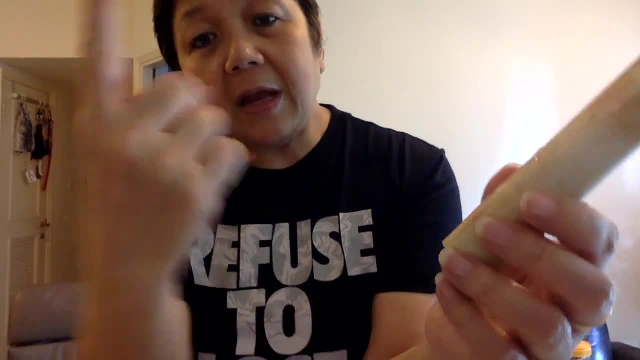 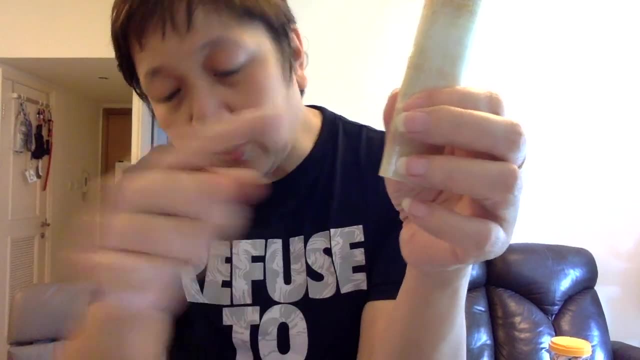 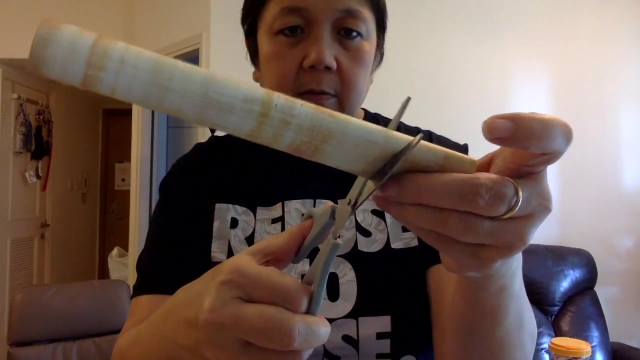 I should, okay, bend a little bit about an inch. okay, see, one, one segment of my finger, okay, one segment on my finger, so I'm gonna cut over here. okay, so I'm cutting, okay, and see, I have a cut over there. okay, so I'm just going to insert. 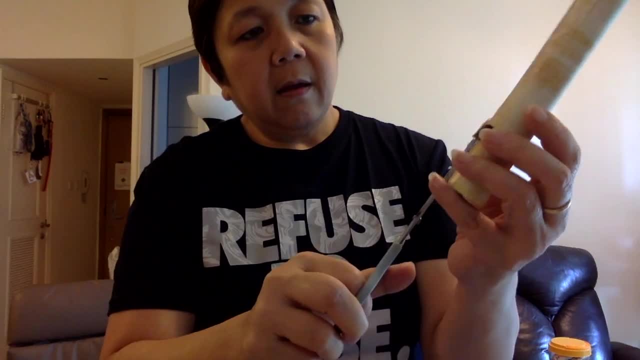 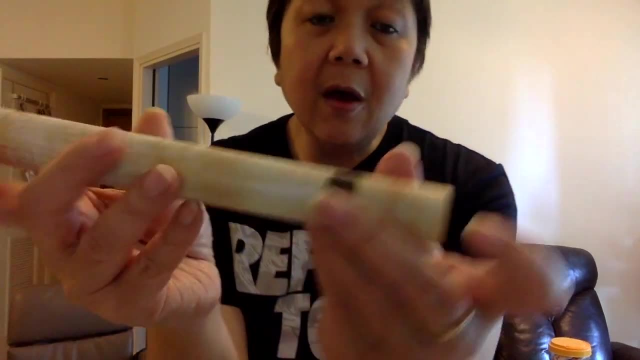 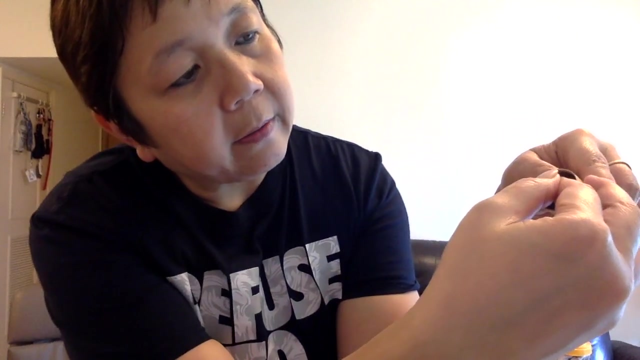 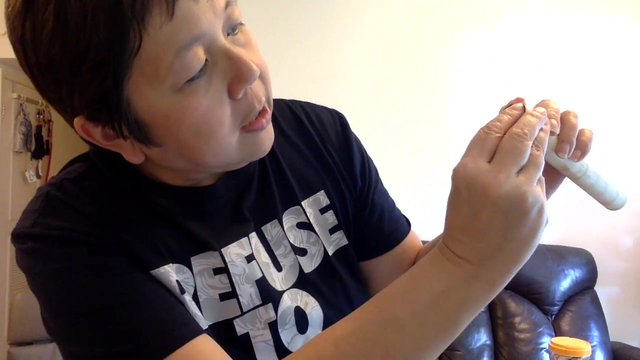 my scissors. and there you go, I have a flap and I cut it done. okay, so now you have an opening here. you want to separate just the top part? okay, so you have an opening here. you want to separate just the top part. okay, so you You need to go all the way, so you only have one layer on top and everything else separated. 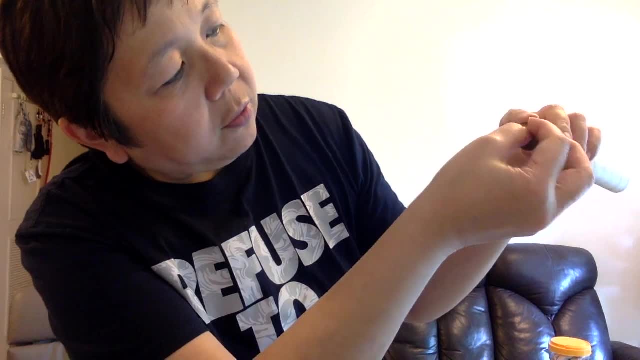 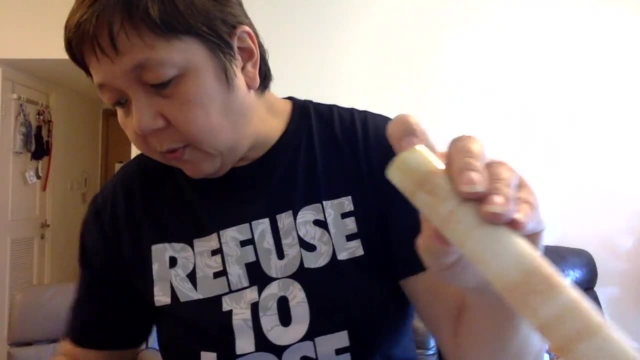 So that's what I'm trying to do. Okay, there you go, See. Okay. So there you go. Only one layer there and separate the rest. And it's easier if you use the scissors: Just insert the pair of scissors. 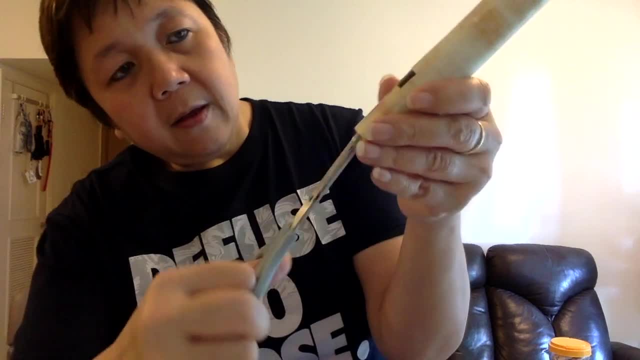 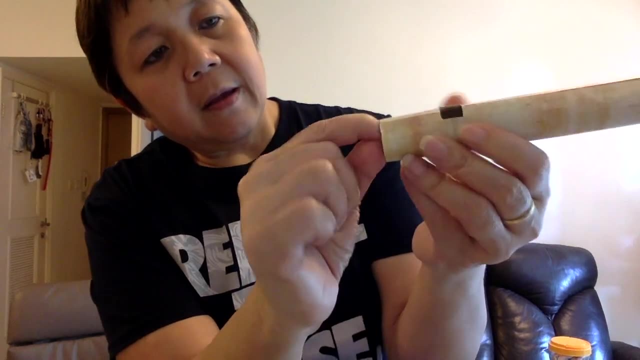 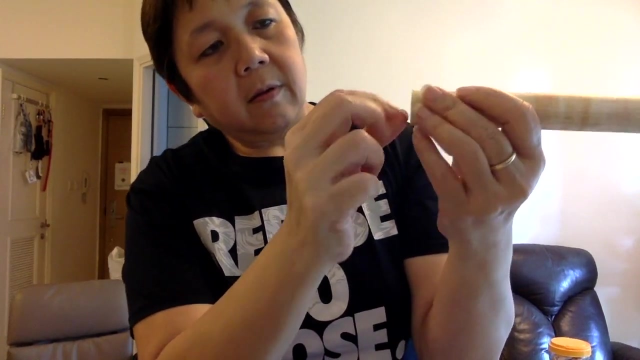 Okay, So that you can separate. Okay, Okay, separate the layer. So there you go. So my layers are now separated And I'm just going to try to make a tiny V shape over here. Okay, Okay, there you go. 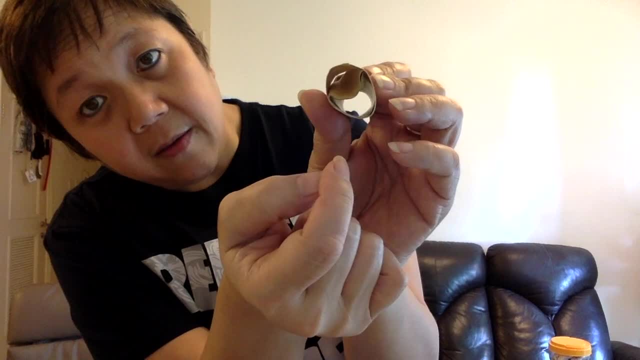 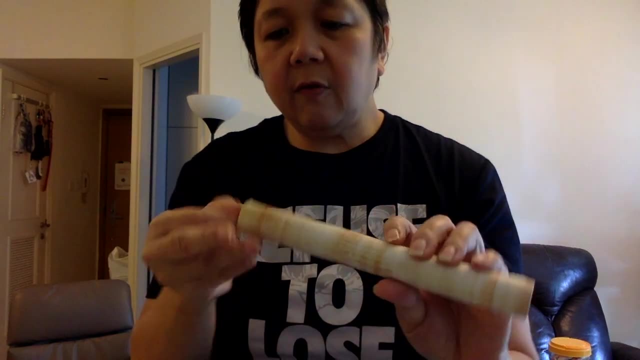 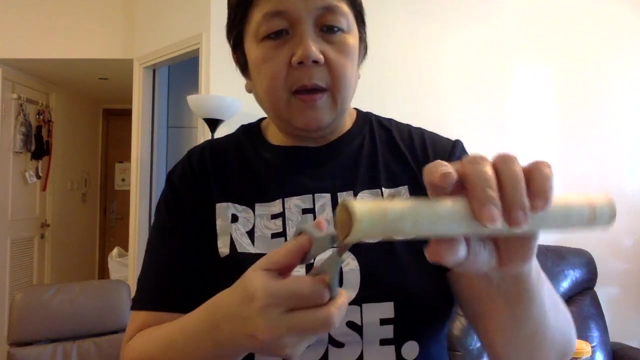 Okay, so I'm just making a V shape over here. Okay, And let's try. Okay, Okay. so it just takes a little bit of fiddling. Sometimes you want to open it all the way here. Okay, So I'm just going to insert my pair of scissors again. 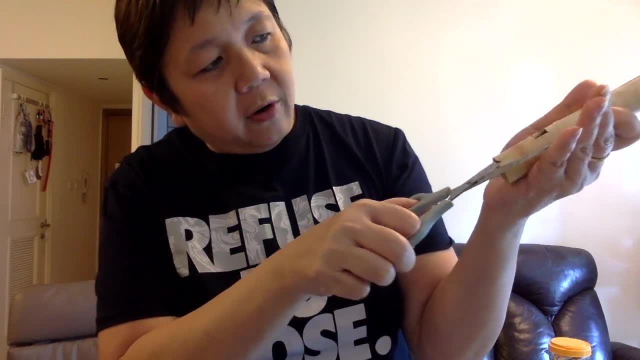 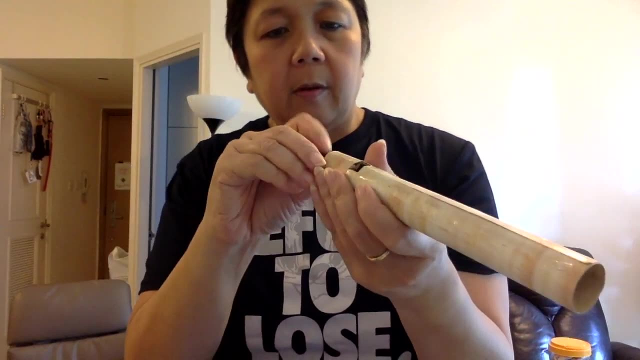 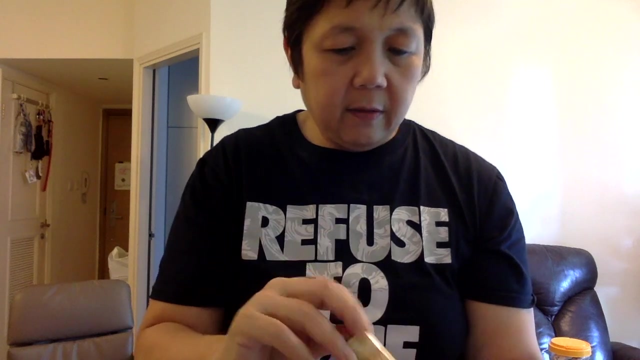 And I'm just going to try to separate it a little bit more. Okay, Just try to separate it a little bit more, Okay, And let's see how that works, Okay. So let's separate it, Separate it, Okay. Okay, let me. 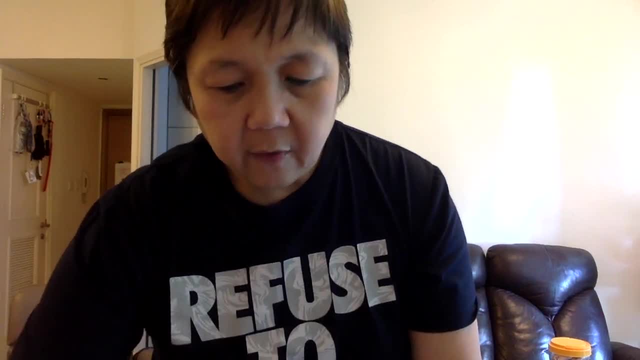 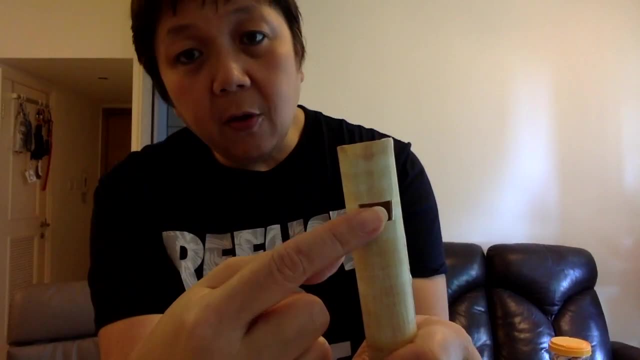 I'm going to try to. I'm going to make the hole a little bit bigger, Okay. So let's try it. I'm going to make it bigger, Okay. So I made the hole a little bit bigger And you can see the hole inside. 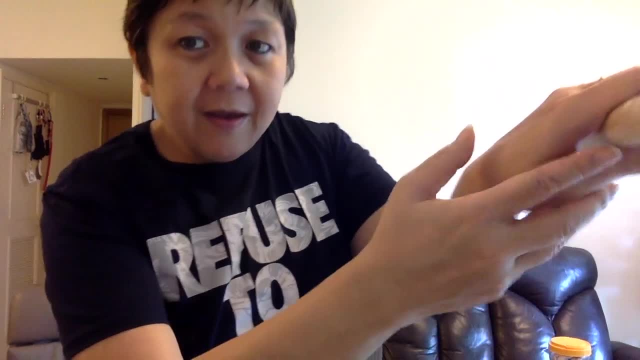 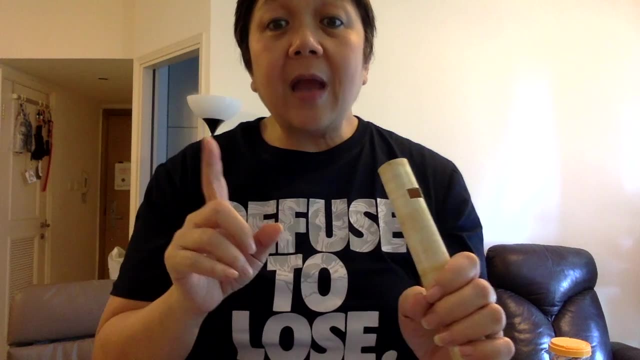 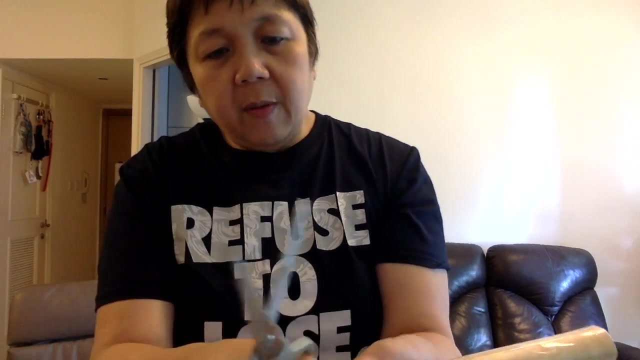 Okay, I made it a little bit smaller, So you need to try to fiddle with the hole, Okay. Okay, now I'm going to add additional holes here. Okay, I'm going to cut. Okay, So I'm just going to press this together. 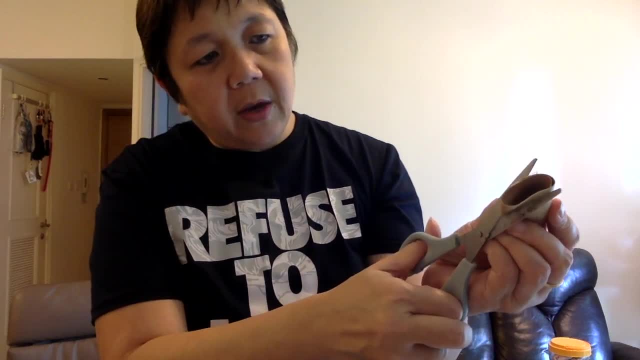 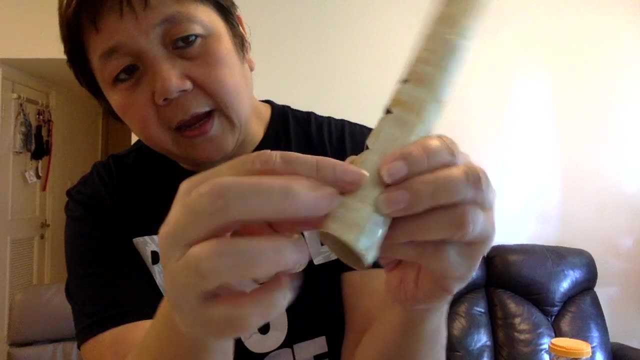 And just make a V cut. So I made three holes already And I'm just going to add, Okay, One more. I just cut it on an angle Like a V, Okay, And there you go, Remove it. So